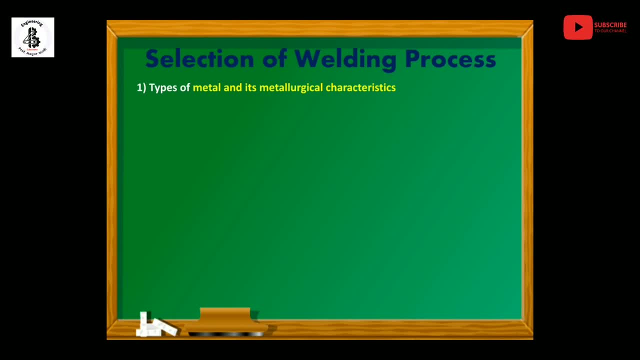 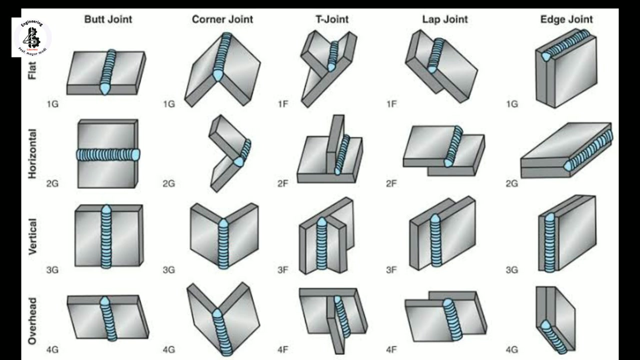 similar, So you can take care about the metallurgical characteristics of both the metals, as well as the filler matter, Then types of joints, its location and welding positions. So basically, into the welding process it will be the butt joint, left joint corner. 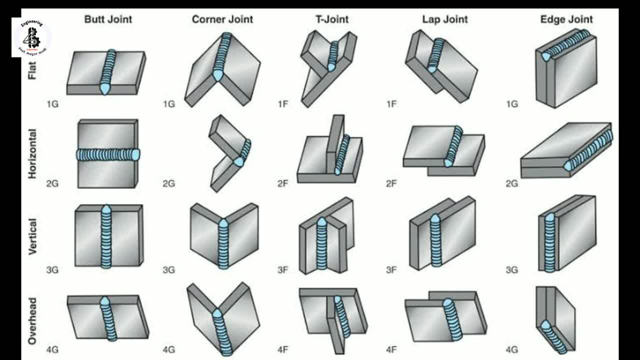 joint T joints and fillet kind of weld, And its location wise it will be the 1G position, 2G position, 3G positions and 4G positions And into the location wise. one more thing: flat position, horizontal positions, vertical. 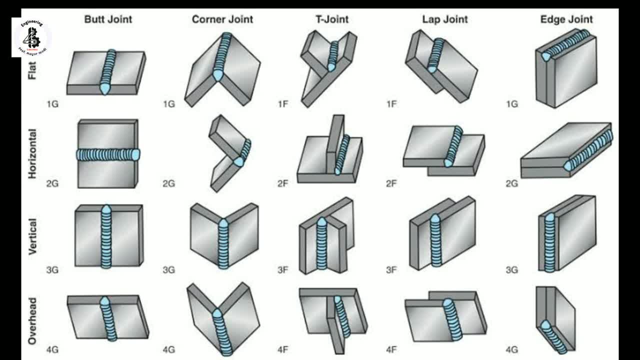 positions, or you can say difficult one, and that will be the overhead positions. So that will be all regarding for the welding positions. So if you want to learn in details for the types of joints and its location and welding positions, so you will find a link in my description. 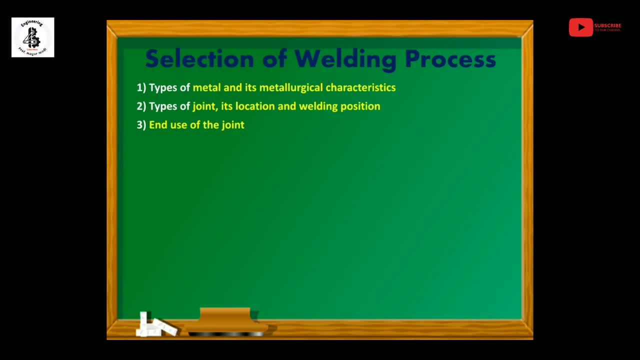 Then after end use of the joint. So which kind of under the loading conditions of your applications. So, as per your requirement of the applications, you will select the various welding processes, Cost of the productions, So each and every products that will be having a low cost without compromising with its performance. 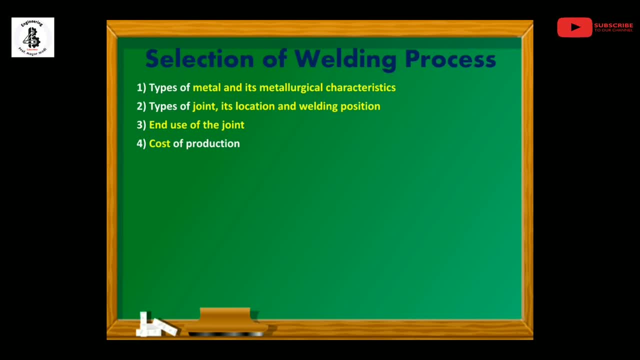 So we are preferring with the low cost of the production. So that's it. So the last one is the structural size. So which kind of size of your jobs? So, according to its strength required, its structure, or you can say geometry requirements. 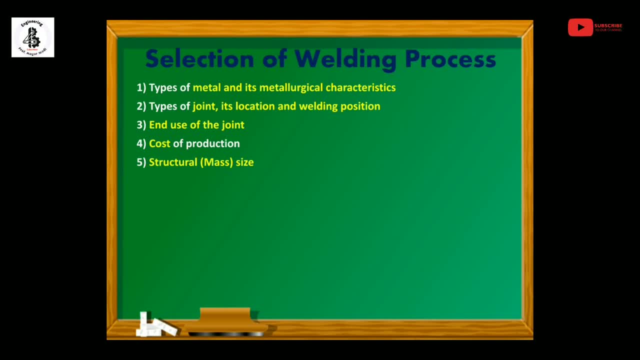 you would like to select the various welding process, So with the minimum cost and it will be having a sound welding, So such kind of process is being selected. So it will be also considering as a mass size or structural size, Desire performance. So welding is considering as a permanent joint. 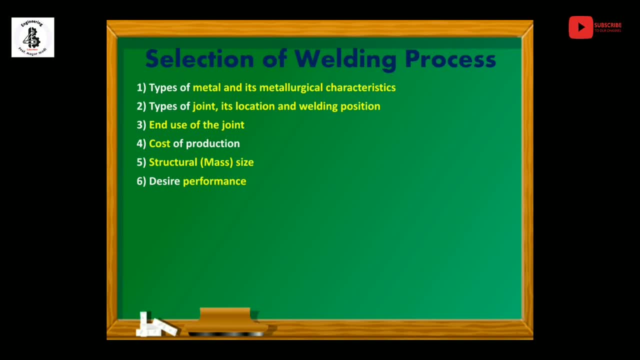 So, according to its definition wise, there will be some desire output is required into the under the loading conditions, So that under the loading conditions, it may be high temperature, pressure, tensile load, compression, load, fatigue loads. So, according to requirement of its desire performance, it will be the selection of the 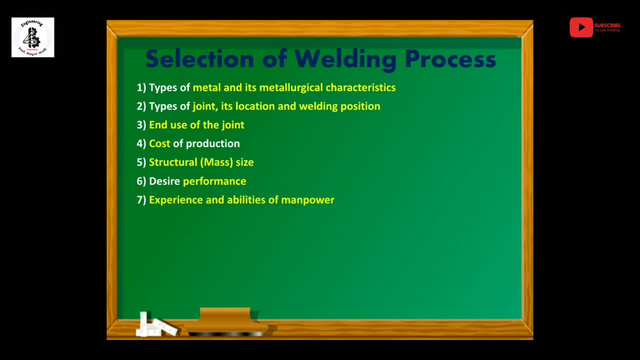 welding process: Experience and ability of the manpower. So this is what we are going to talk about in this video. So nowadays, for the critical applications, there will be the major requirements- experience and abilities of manpower. So you can also considering as a skill is being required to performing the sound weld. 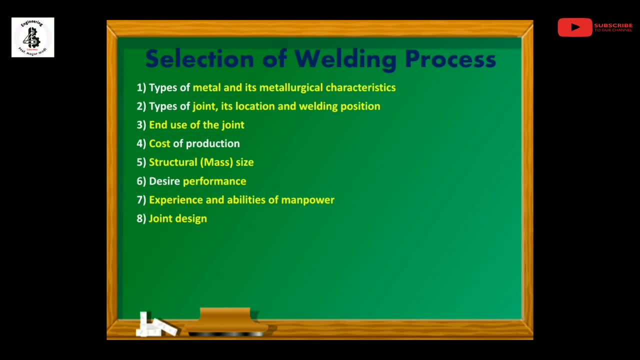 Joint design. So once again that would be depends upon the geometry strength of the weld. So it will be the single side, double side, single fillet, double fillet according to its requirement of the geometry. So that will be having a different joint designs. 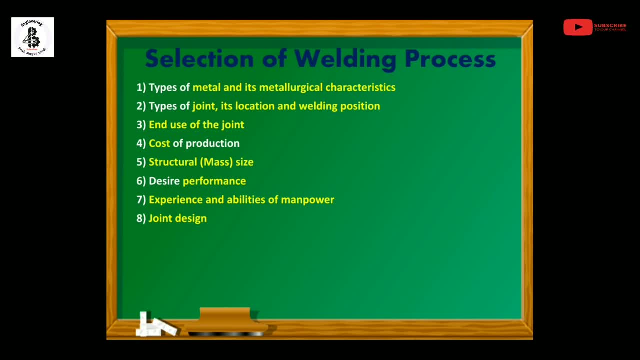 So, according to its complexity of the joint designs, it will be also selection of the welding process. Accuracy of assembling requirements. So, as per the definition of the standardization accuracy that will be the necessary conditions for assembling of your such a components with the another components. 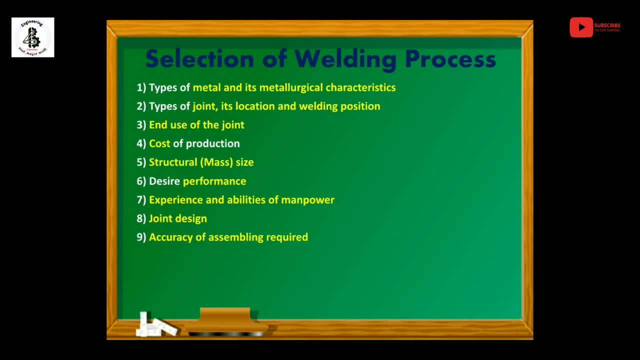 So that will be also important Part for the selection of the welding process, Welding equipment available. So, once again, which kind of resources is being available for us, So that resources with the minimum cost and without compromising with the performance? So you would like to select such kind of welding process. 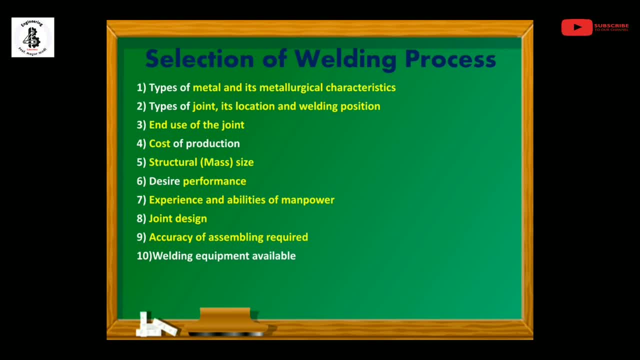 So that will be the one important part and it will be the welding equipment available. So, basis on to the availability, Then work sequence, So as per the American society, and that would be the WPS, or you can say welding procedure standards. So how would like to make a sequence for manufacturing of such components? 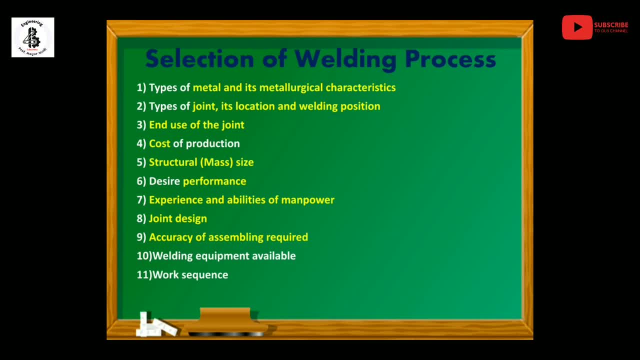 So according to that it will be also one part of the selection of the welding process and that will be the work sequence. After that: welder skill. So nowadays it will be the highly requirement of the skill of the welders. So that will be the work sequence. 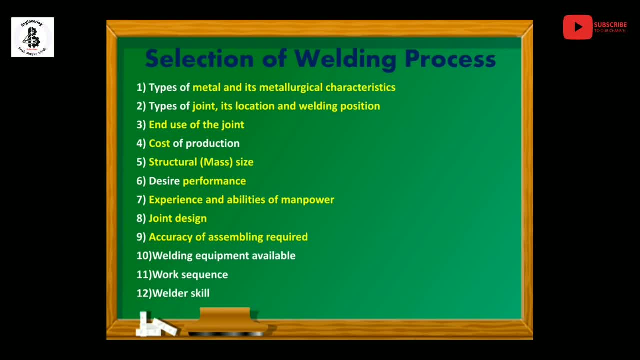 For the critical applications like boilers, pressure vessels and various kind of heat exchangers, And nowadays for the low density and high strength materials, it will be used into the aerospace missiles. So at that, critical applications, there will be the requirement of the skill of the welder.